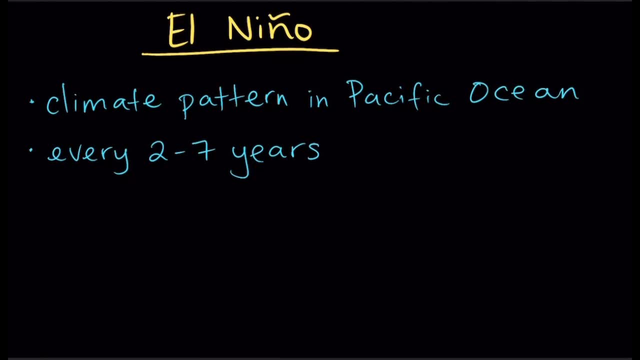 Nino can bring about heavy rainfall and flooding. it can also cause severe drought. So it's really important to note that El Nino is not just a storm. It's also a climate pattern that takes place all year long, So it's important to note that different regions around the world experience 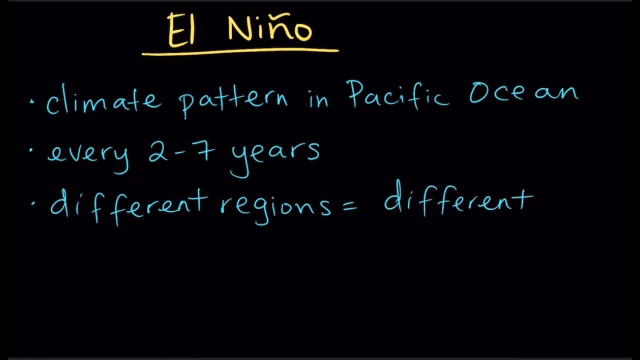 different effects of El Nino, And we'll see a few examples of those. So sometimes an El Nino year is actually a little bit helpful and might bring about some much needed rain, But other times, bigger and more severe El Nino events can bring devastating weather events all across the globe. 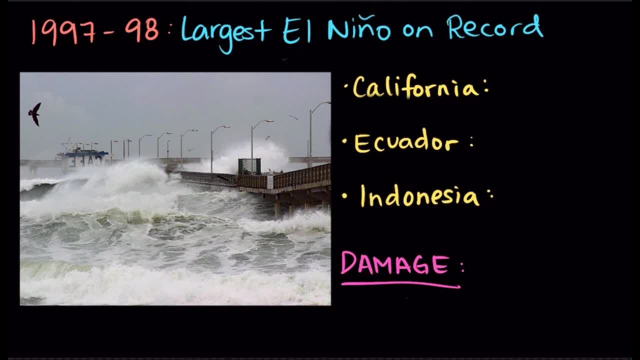 So we can look at the different effects by looking at the biggest El Nino on record during the 1997 to 1998 season And we can see how different regions were affected. So for example, in California we saw very destructive mudslides. In Ecuador there was heavy rainfall. 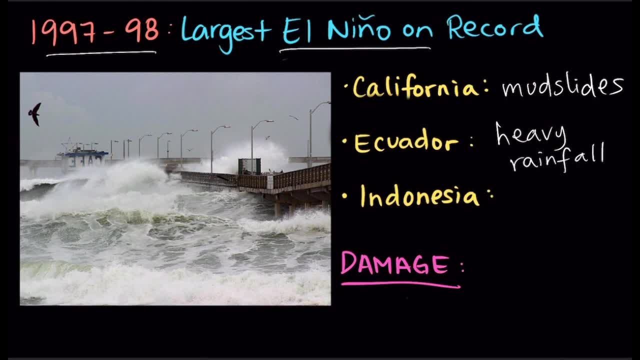 And in Indonesia there was actually extreme drought and fire And overall this El Nino event was really large and very destructive. There are estimates of about $36 billion in damage to infrastructure. So you might be asking yourself: how can the same? 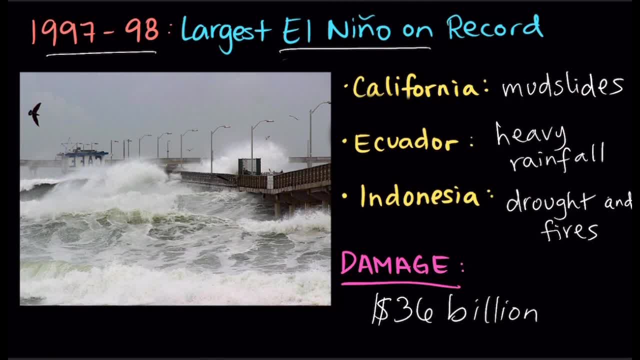 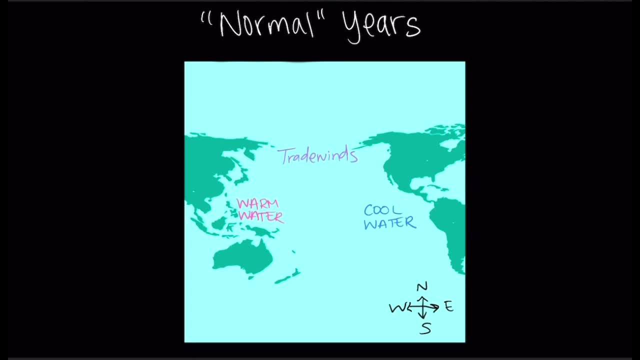 climate pattern cause such drastically different effects around the globe. So to understand this better, we have to look at what a quote- unquote- normal year looks like. So this is a map of the Pacific Ocean, And normally there are trade winds that are pushing. 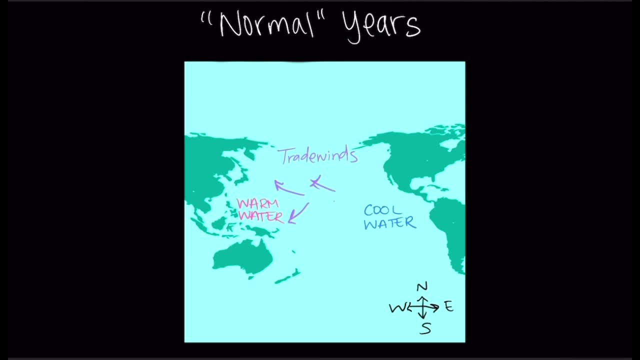 warm water towards the west, so towards Asia and the Pacific Islands, And warm water accumulates on this side. On the other side, on the east side, near Central and South America, we have an accumulation of cool water, And this is also due to a process called upwelling. 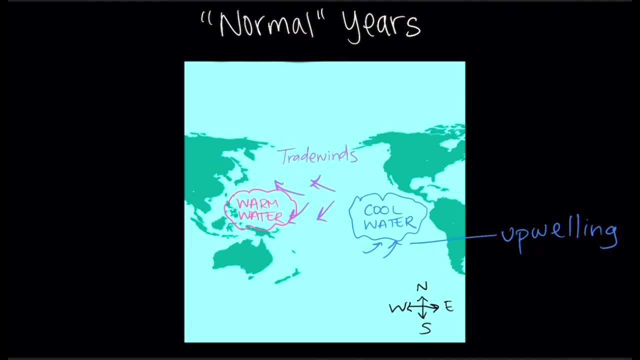 Where cold water from the bottom of the ocean is pushed up, And during these conditions in general, you would see less rain on this side, While you'll see more rain on this side. Okay, so now let's look at what changes during an El Nino. 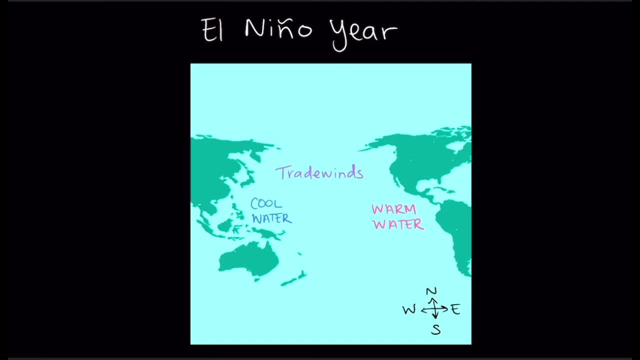 year. So during an El Nino year you still have trade winds pushing water west, But they're much weaker And that's the key here: That your trade winds are weakened, Which means less water is pushed towards Asia and the Pacific Islands. So, compared to a normal year, 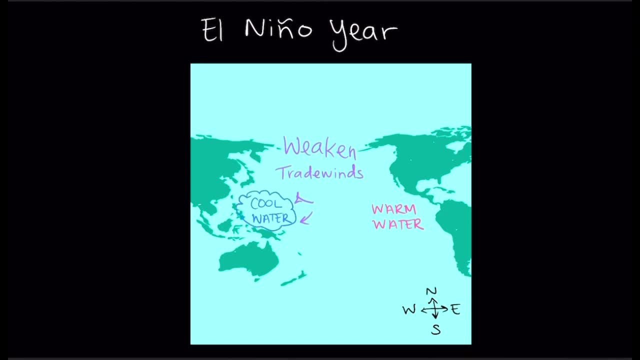 you actually have cooler water that starts to accumulate on this side of the Pacific Ocean. Meanwhile on the other side, since less water is being pushed away from Central and South America, you get more warm water accumulating. So now you can think back to those South American fishermen. 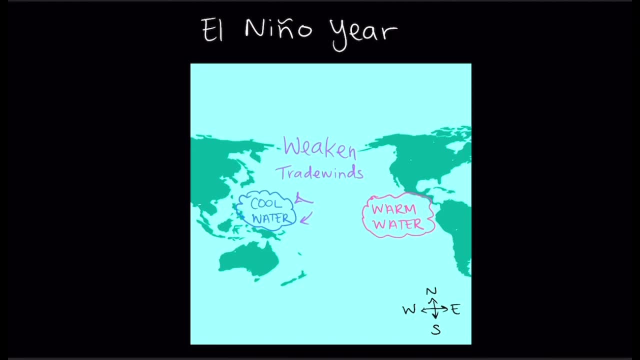 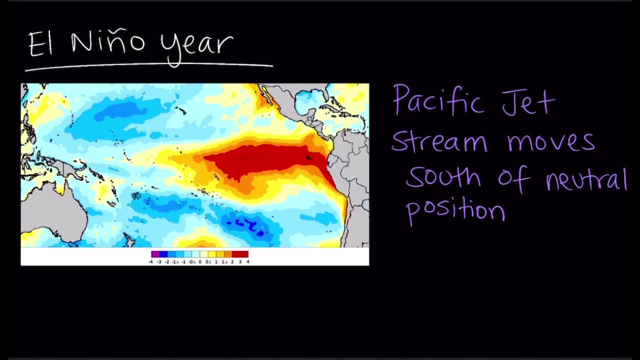 and why they were experiencing warm water along their coasts during an El Nino year. So this map does a really great job of showing the temperature gradient and how this warm water is staying along the coast of Central and South America during an El Nino year. Meanwhile, you 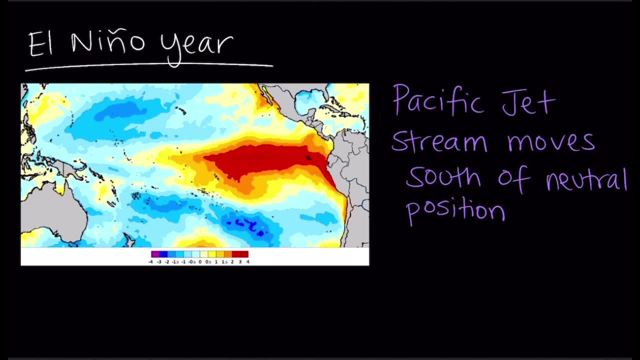 have cold water accumulating towards Asia And this causes a lot of changes that affect weather patterns. So in the US the Pacific jet stream moves south of its neutral position And because of that we start to see that the northern US and Canada are actually warmer and drier than they usually are. The US Gulf 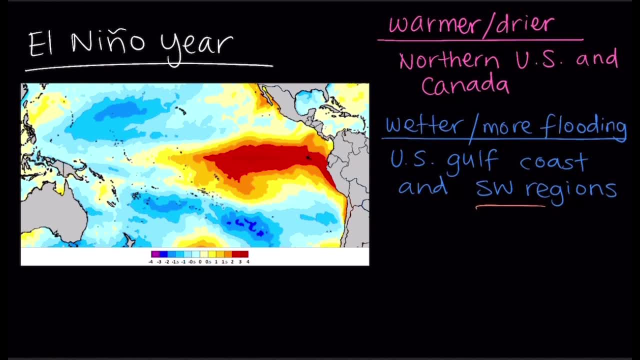 Coast and southwest regions of the US are wetter and at a more increased risk for flooding, And so the US and Canada are actually warmer and drier than they usually are. South Asia and the Pacific Islands experience warmer and drier conditions that lead to drought. 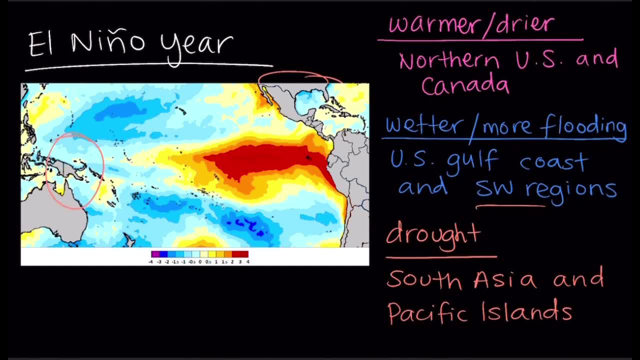 on the other side of the Pacific Ocean. So now you start to see how one event, El Nino, this one climate pattern, can cause both flooding on one side of the Pacific Ocean while also causing drought on the other side. And finally, we'll end with La Nina, because you might hear this: 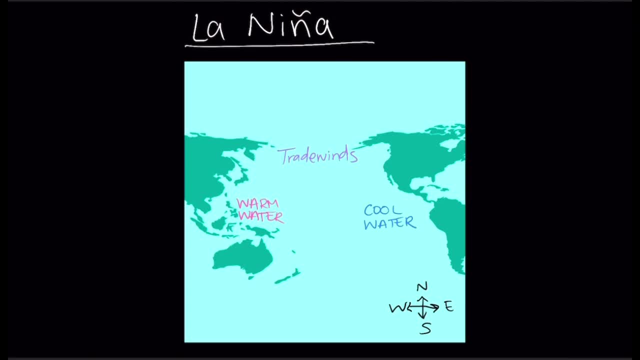 come up too when talking about El Nino. So La Nina is essentially the opposite. So if you've got El Nino down, you can start to understand what happens during a La Nina event. So in this situation, our trade winds are getting stronger than our normal years, So they're pushing water.